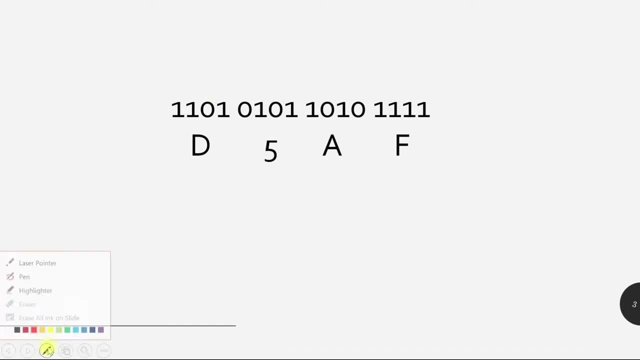 You know from before that the hexadecimal values are ranging from from 0 till 9.. 0,, 1,, 2,, 3, then up to 9.. After 9, we have the letters a, which is representing 10.. b, which is 11.. c, which is 12.. 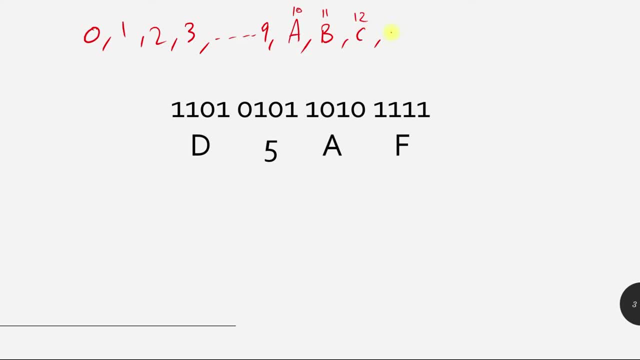 d is 13.. e represents 14. And then f, which is the last digit here in hexadecimal number system, which is representing 15.. As you can see here screen four digits of binary code is represented by only one hexadecimal digits, which is easier for humans to understand than binary, as it is. 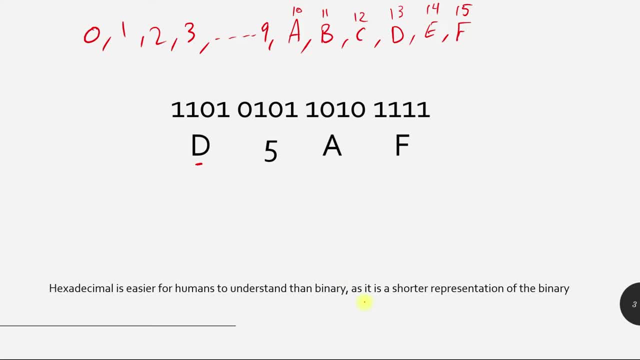 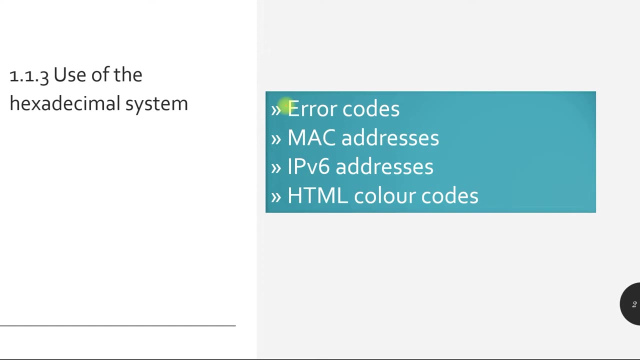 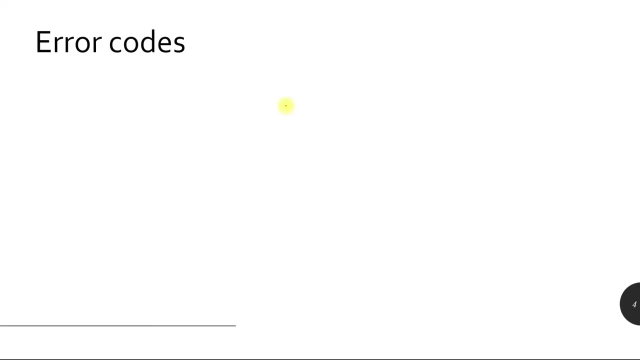 shorter representation of the binary code. which one is easier? definitely the last one, which has only four hexadecimal digits. now let's look back at the use of hexadecimal system: error codes, MAC addresses, IP version 6, HTML, color codes. let's start with the first one: error codes. we know sometimes when we are 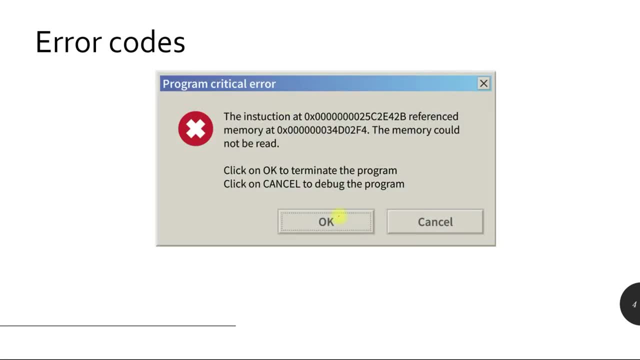 using computers, error messages like this one might appear for you, as you can see here this error message: program: critical error. some programs might cause an error in memory and this is represented, as you can see here, by hexadecimal values: 25C2, E4 to B. reference it also in memory as in hexadecimal values. imagine that if 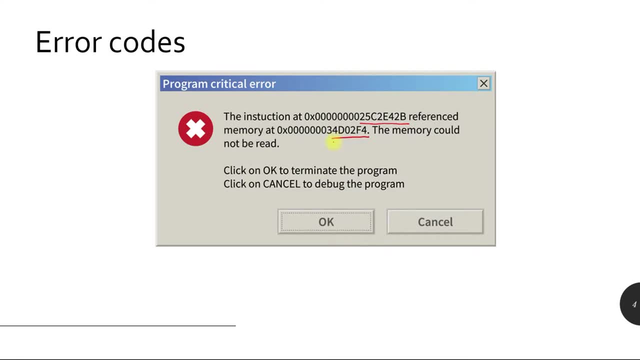 this value. here this number is represented by a binary number, so this will take longer space and it will be very hard to humans to understand and read error codes. these numbers refer to the memory location of the error, are usually automatically generated by the computer or the operating system. 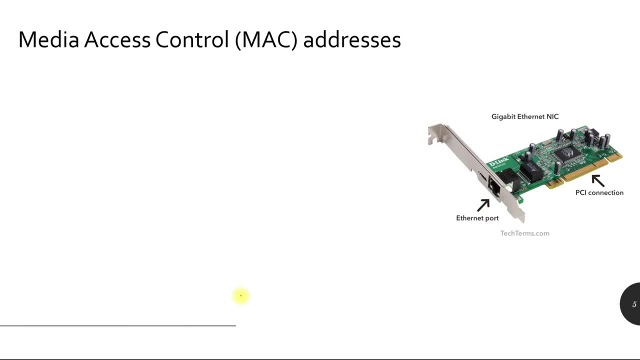 you can also use the MAC addresses here also is which is known as media access control. media access control, or MAC addresses, refers to the number which uniquely identifies a device on a network. the MAC address refers to the network interface card, NIC, which is part of the device. every computer, every smartphone. 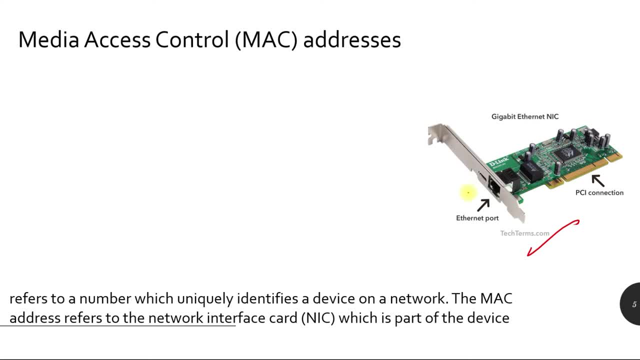 connected to a network must have a network card, network interface card, NIC. in desktop computers the card looks like this one. definitely inside the laptop or smaller devices the NIC card is much smaller than this one. as you can hear, you have Ethernet port where you connect the network cable and MAC address is. 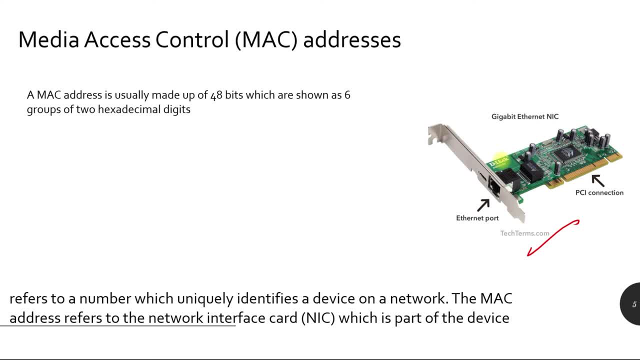 usually made up of 48 bits, which are shown as six groups of two hexadecimal digits. so you have six groups here. every group is denoted and then each editable number is given in specific animals. all 7 digits in the array. so we're turning to yarn forbricks, values by performs we have. each editable value is сейчас. 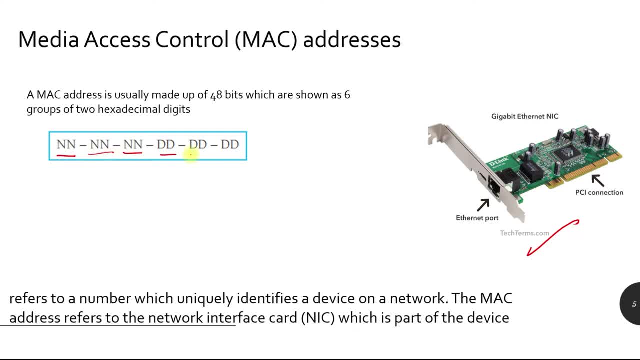 contains two hexadecimal digits. this is just representing hexadecimal grouping, six groups. as you can see here, each group consists of two hexadecimal digits, the first three groups. here NNNN is to identify the number of manufacturer of the device. this device is made by a specific manufacturer and 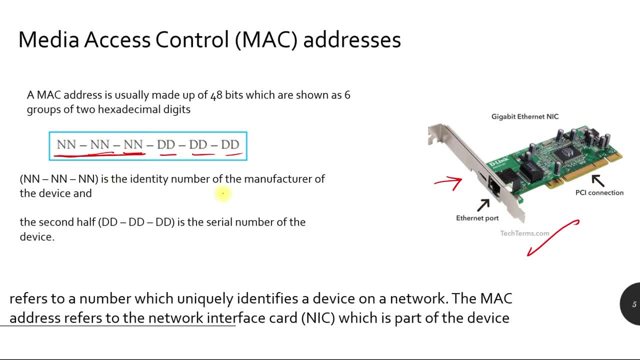 every manufacturer has its own unique manufacturer number. and then the second group, the second three groups. here is a serial number of the device. each device has a manufacturer ID and then a serial number specifically for this device. for example, Dell computers, Dell company, has the hexadecimal values as zero, zero one. 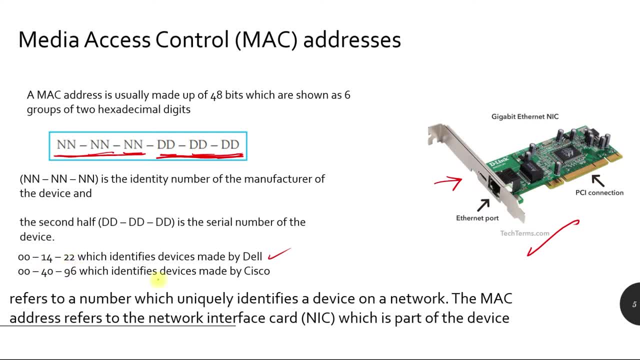 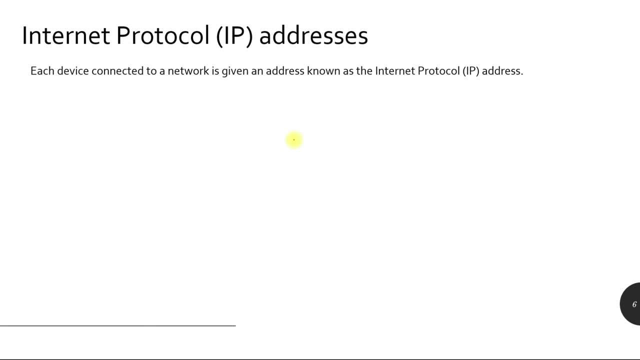 four, two, two Cisco computers. Cisco devices also have the value of hexadecimal 004096. The third application or the third use of hexadecimal number system is IP addresses or internet protocol. Each device connected to a network is given an address known as IP address or internet protocol. 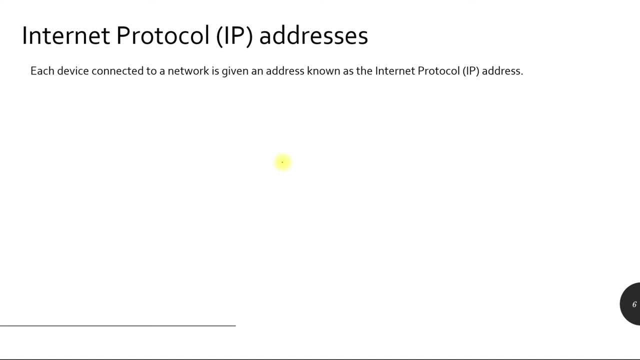 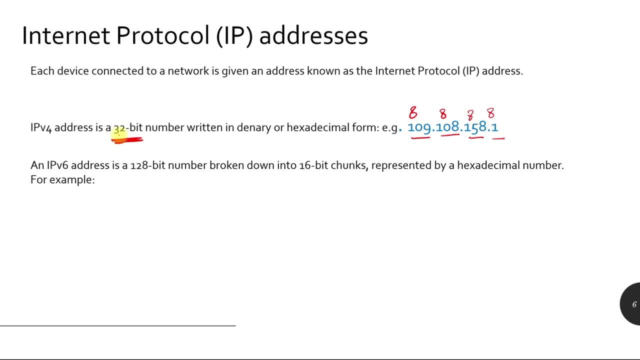 The recent and more advanced IP version 6 address has more number of bits- 128 bits Will be broken into 16-bit chunks represented by a hexadecimal number. For example, this value here, Every chunk here, is representing 16 bits, since they are 4 hexadecimal digits. 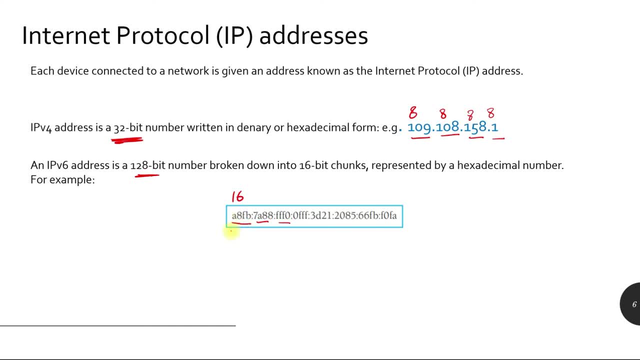 And every hexadecimal digit is represented by a hexadecimal number. So in total, every chunk here is representing 16 bits. Imagine if we wrote this in a binary value. this will take 16 bits, So 16 bits, and then 16,, 16,, 16,, 16 bits, and so on. 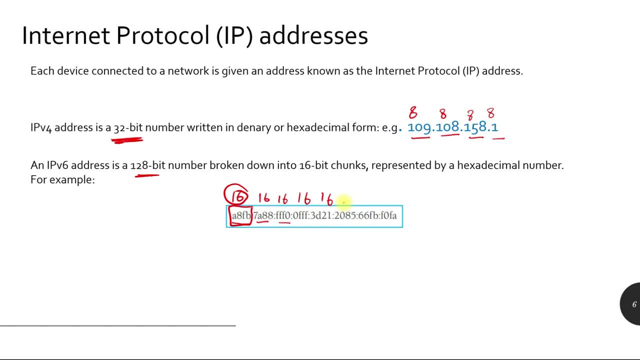 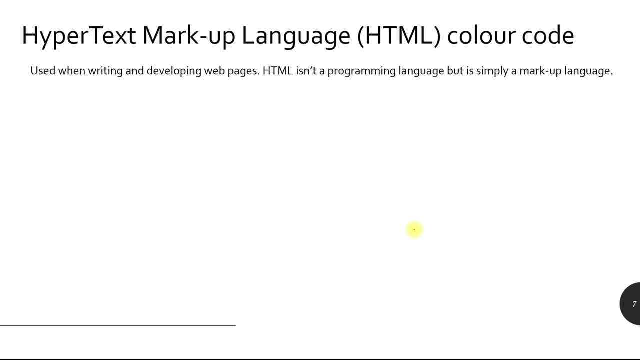 So rather than these short hexadecimal values, it will be very long, up to 128 bits. Note that IP version 6 uses a column here instead of the dot in the IP version 4. This one is much recent than the IP version 4. The last application, last use here of hexadecimal number system is the HTML color code. 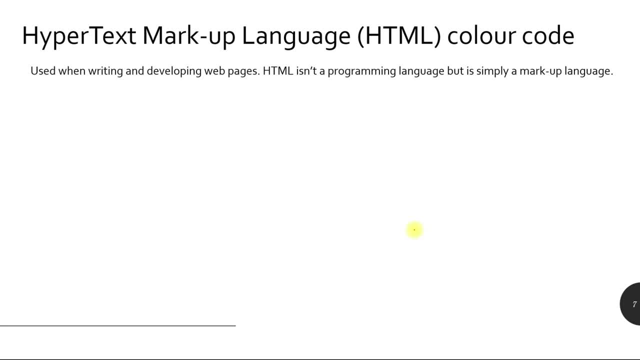 Hyper Text Markup Language used when writing and developing web pages. HTML isn't a programming language, But is simply a markup language. When you have a website, This website might have some like, for example, picture A table. here It might have some text. So marking up the spaces on the web page is known as marking up. 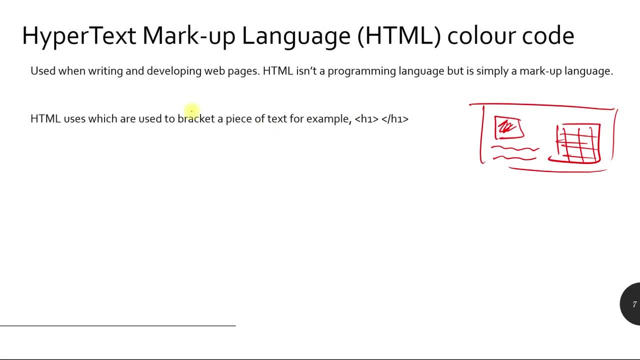 HTML uses, which are used to bracket a piece of text, For example h1, and then close the bracket with h1. These are known as tags. Instead of representing the colors in a long binary number, They can be represented in an easy way using hexadecimal digits, As follows: